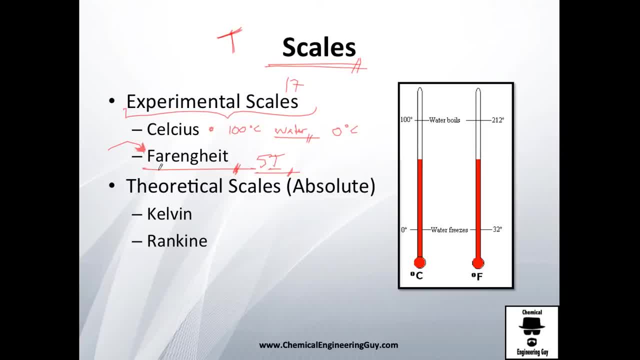 that sense they have a better reference, but actually, well, we're going to see that in the next slide. Then comes the theoretical scales, which are absolute, and these ones are more, let's say, thermodynamically important or relevant, because they are talking about the zero or the zero. 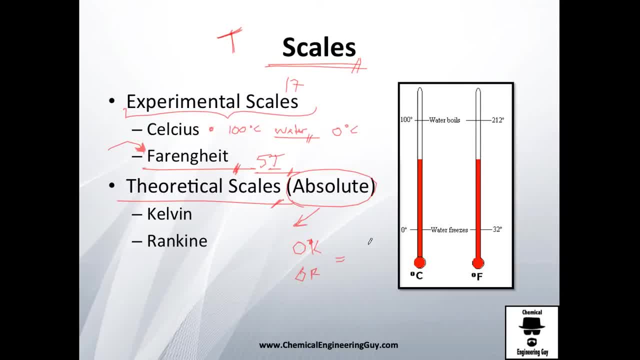 kelvin or zero ranking actually are the same, because it's when the molecules stop at all. and I think it makes a lot of sense because when the molecule has no average kinetic velocity, which is this, When they stop moving, they have zero value, and that's, you know, in mathematics, zero is. 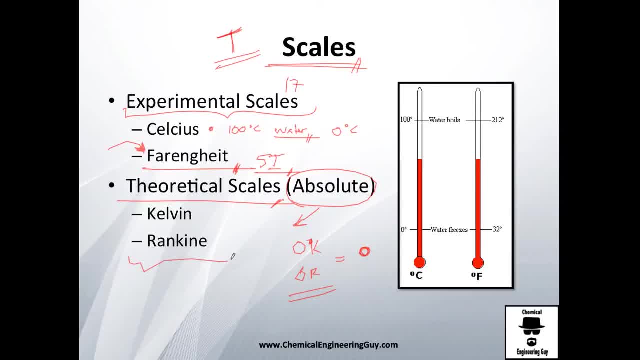 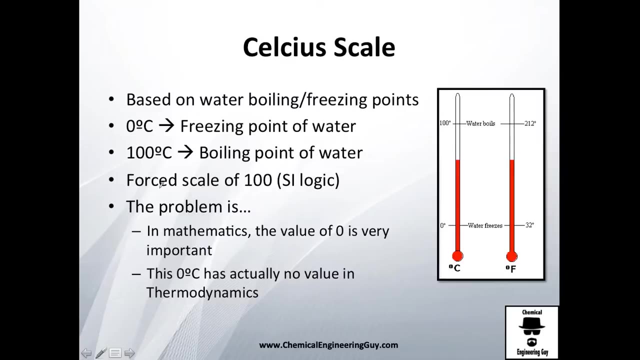 a very special number, and thermodynamics in these scales. this is also a very specific number. If you use zero Fahrenheit and zero Celsius, well, they don't make that much of sense. we're going to see that later More on the Celsius scale. sorry about going very fast, but I wanted to give you the Celsius. 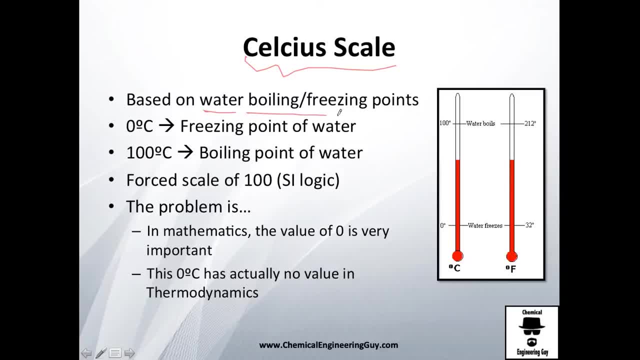 scale Right now it's based on the water and the bailing, boiling and freezing points of it: zero Celsius freezing point, 100 Celsius boiling point, and the user who invented it- probably Celsius- forced the scale to be a hundred, let's say 100 degrees, because he could actually 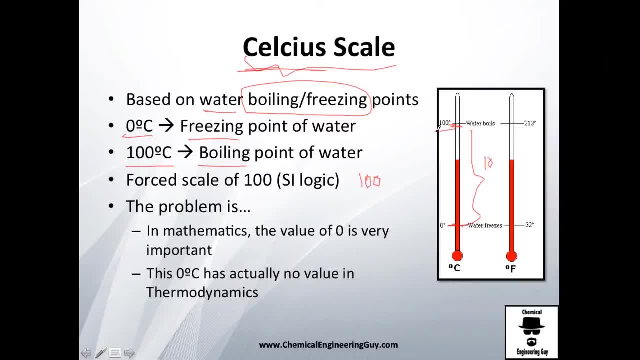 use one or ten, but he decided to use 100. or even he could use 1000, but he chose to be 100.. That's good. I think that this is very logic for the international system. The problem is that in mathematics, the value of zero is very important, as I told you before. 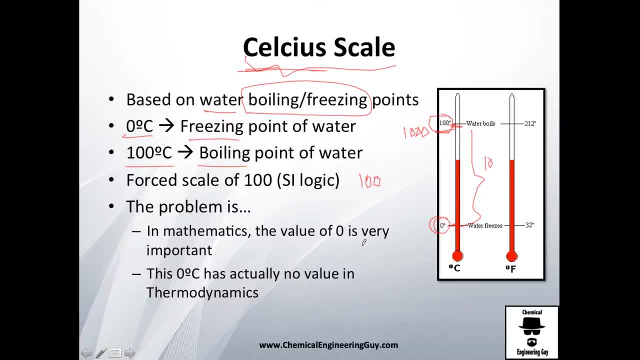 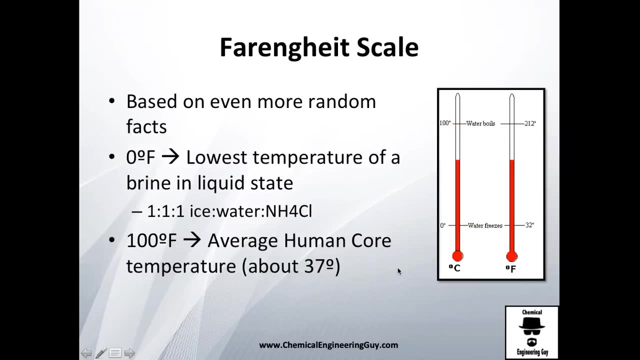 so T zero in thermodynamics or T zero Celsius is not that relevant. If you're speaking on water, okay, maybe it's the freezing point of water, but if you're using other temperatures- I mean other substances- it does not make sense at all. Then comes the Fahrenheit scale. 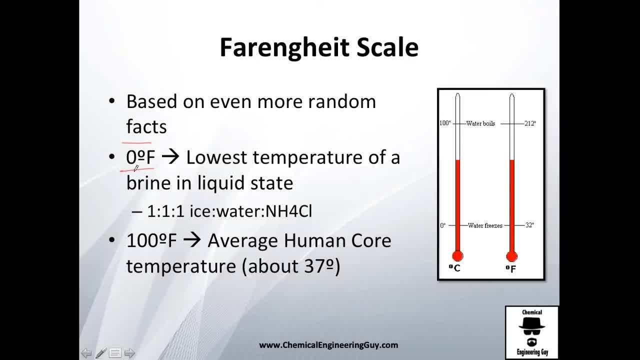 It's based on even more random facts. Let me tell you: zero Fahrenheit was the lowest temperature of a brine in liquid state. So this guy Fahrenheit actually German. many will think it's American or British, but not. he was German. He choose that. he will mix one to one to one. what do I mean with that is one kilo of ice. 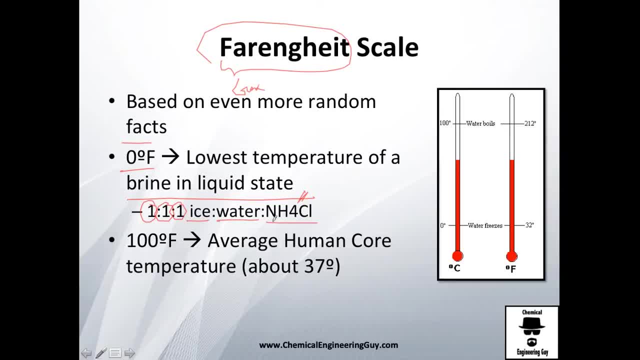 one kilo of water and one kilo of this salt, which is ammonium chloride. He mix it in a bowl and then he choose that, whatever the temperature was there, he will name it zero Fahrenheit, which will be something around here. Zero Fahrenheit, I think, is about minus something degrees Celsius. degree, sorry, and okay, that's. 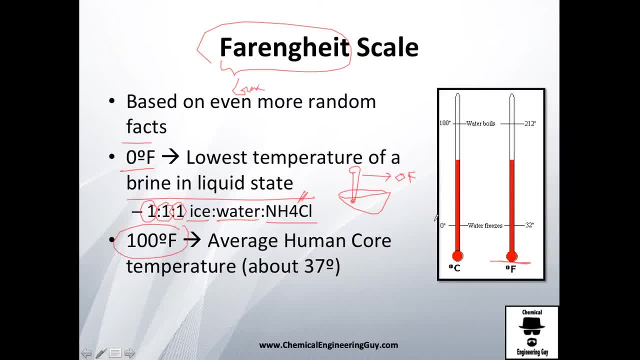 the first one. Then he told I need another hundred scale. so because probably zero- and one hundred was pretty famous scale, He choose it. Fahrenheit also choose it, but he did not choose the water boiling. he choose the average human core temperature, which is about 37 Fahrenheit. 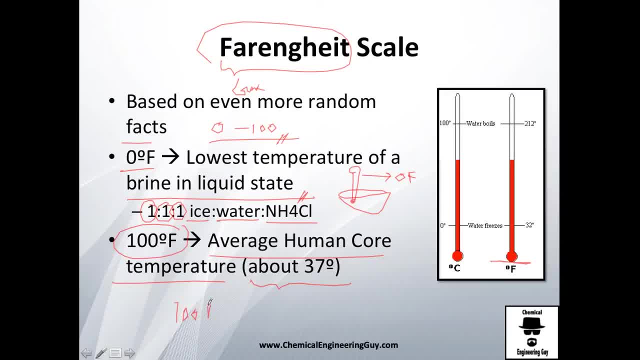 So probably you are between zero a hundred Fahrenheit. you are healthy. you are low, you are not healthy. you are maybe having hypothermia, and if you have higher temperature in your body you're probably sick with fever. So that's a good one. But once again, 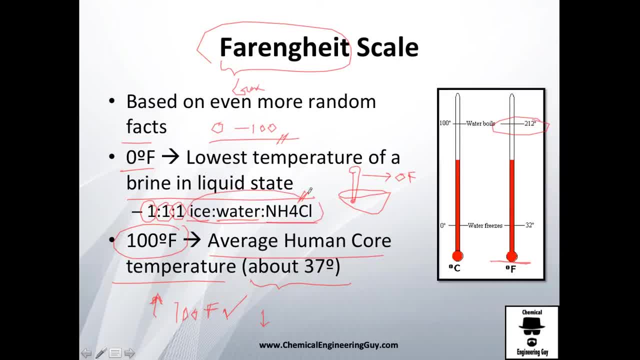 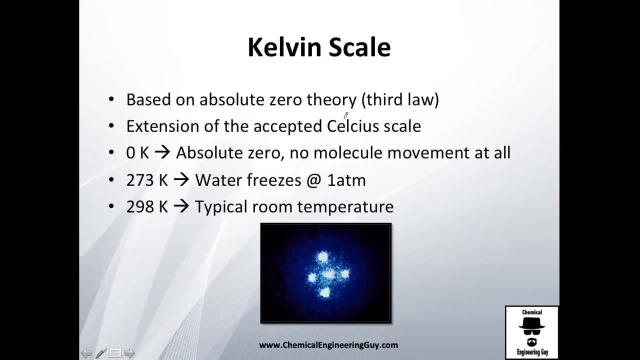 The body, the human body, and this random salt, ice, water and ammonium chloride mixture does not make sense at all in thermodynamics. So eventually Lord Kelvin came and this guy was totally into thermodynamics. he actually got pretty awesome results in that He choose his Kelvin scale and base it on a very thermodynamically important concept. 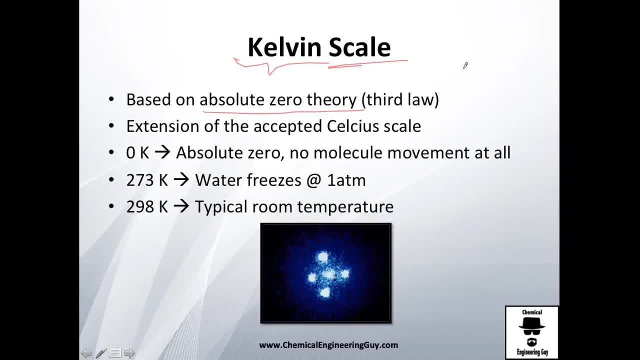 which was the absolute zero theory. What does that mean? essentially, that gases have a lot of movement, then come liquid have partially a lot of movement, solids have a little bit moment and eventually, when they achieve zero or no movement, movement at all, this will be the zero or the absolute zero. 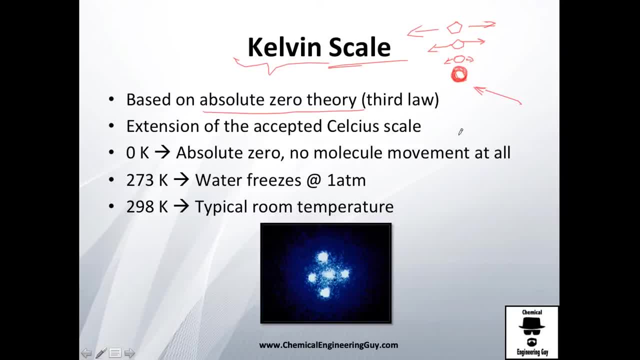 and Kelvin. Lord Kelvin choose this. since he was into Celsius scale, he decided that one Kelvin will be one Celsius, But He will use another reference. instead of using the zero Celsius, he will choose the zero absolute, which in Celsius was minus two hundred seventy three. 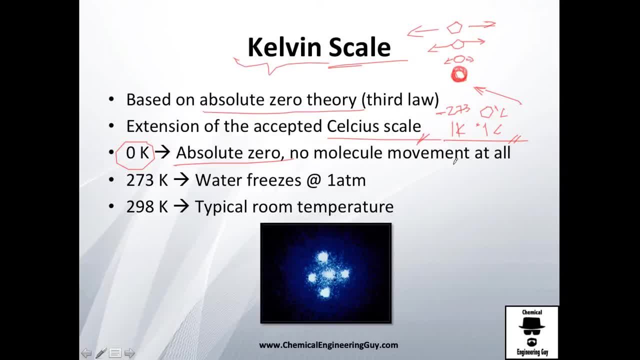 So once again, zero Kelvin is the absolute zero, no molecule movement at all. plus two hundred seventy three Kelvin means zero Celsius and plus twenty five will mean the typical room temperature. So when you hear three hundred Kelvin, Hopefully you get the idea. It's about twenty seven Celsius, which is not that warm. 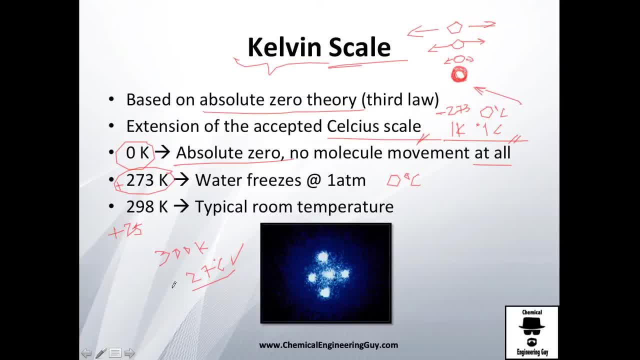 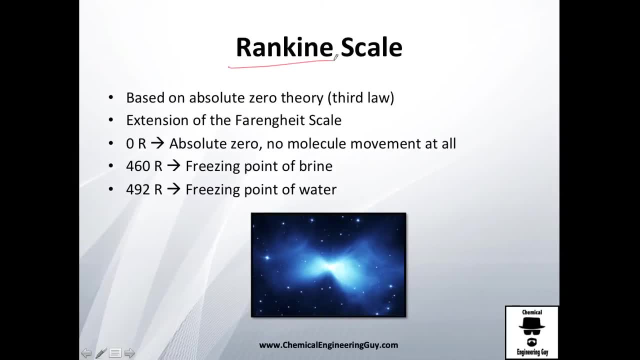 Maybe Europeans would think it's warm, but it's OK, It's room temperature, It's awesome climate weather, etc. And then came ranking, which is the equivalent of Kelvin, but in the English system. This guy was also into Fahrenheit scale. He made the same assumption. 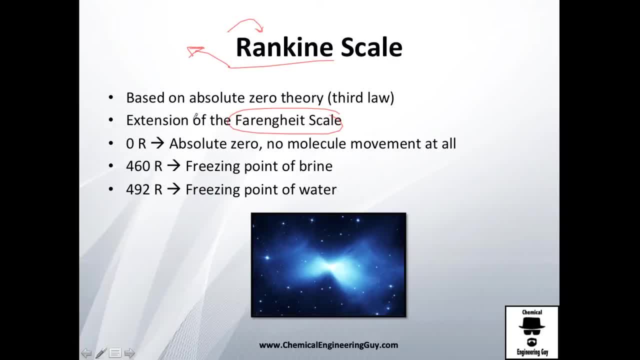 He said maybe. well, if Lord Kelvin did that, Why wouldn't he? I do that in my system. So he used also the absolute zero theory as zero ranking, but a little bit more. one Fahrenheit would be one ranking. So it's essentially the same. 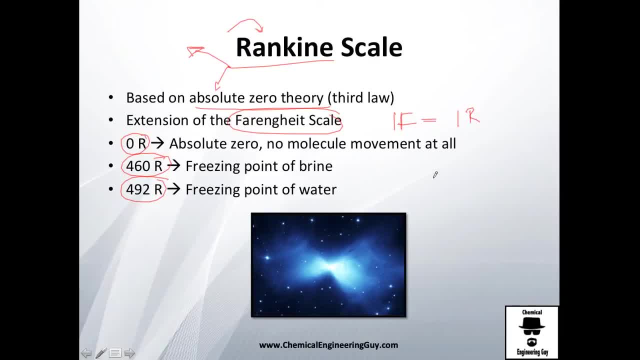 Of course we have another numbers here, and the thing here is that one point eight Celsius is one Fahrenheit, So that's why we have very high temperatures here. Four hundred sixty Four hundred sixty will be the freezing point of that brine he choose. 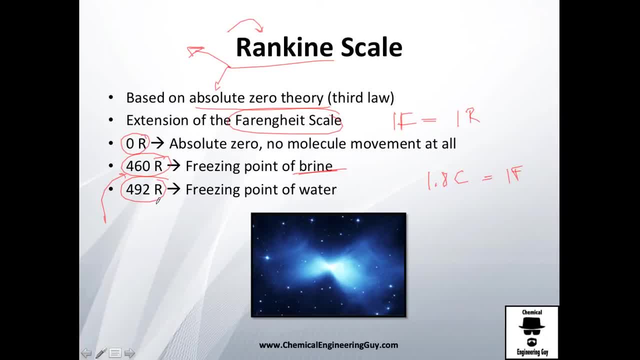 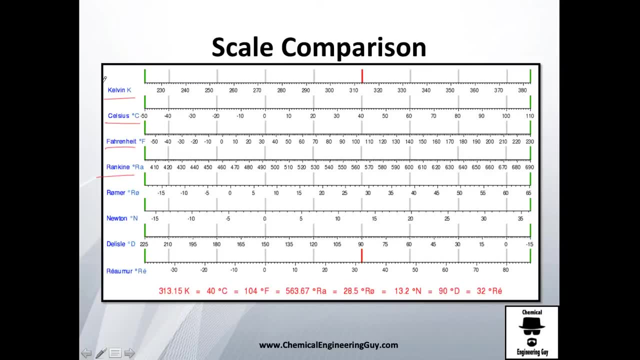 And the freezing point of water will be four hundred ninety two. So let me give you a scale comparison. The ones we choose- Kelvin, Celsius, Fahrenheit and Racking- are the most famous one and the most used one, But of course there are many others. 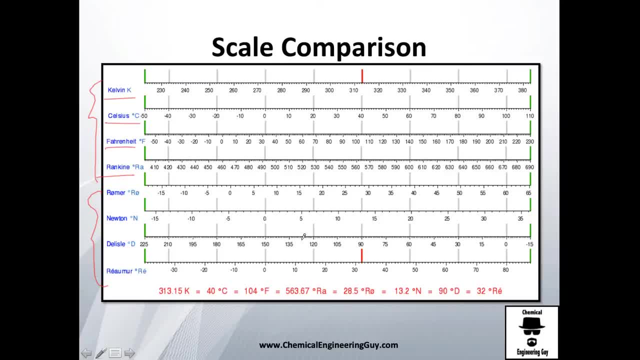 You can have these. maybe pause the video. choose the reference value. I think it's here. If you want to choose- I don't know- Let's choose Twenty five, Twenty five, Thirty, Thirty Celsius. You can find all the values on here. 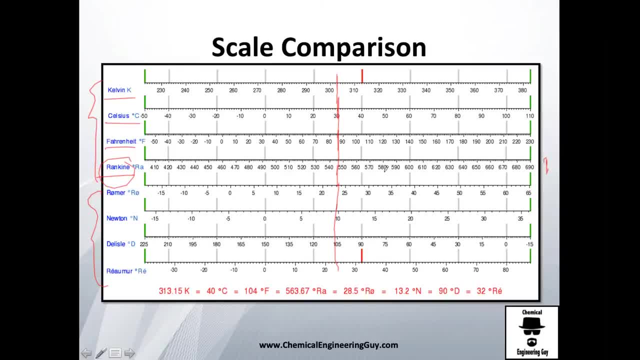 You can see the ranking scale is the one that has very high values. You can find also that the Newton scale, where it has very low values, here Top is thirty five And of course they have different bases, but the important thing is to have the equivalent. 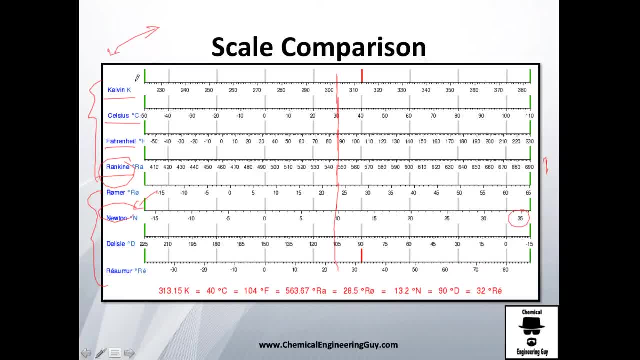 formulas and maybe I'm going to give you later the formulas. You should know them by now, because that's actually, I think, from elementary school or even high school, middle school. You should know that by now. But I'm going to give you to you anyways. 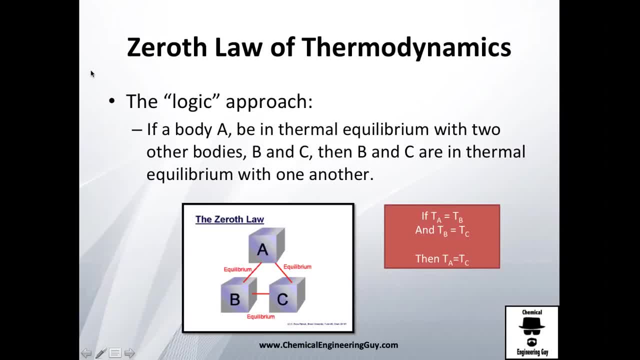 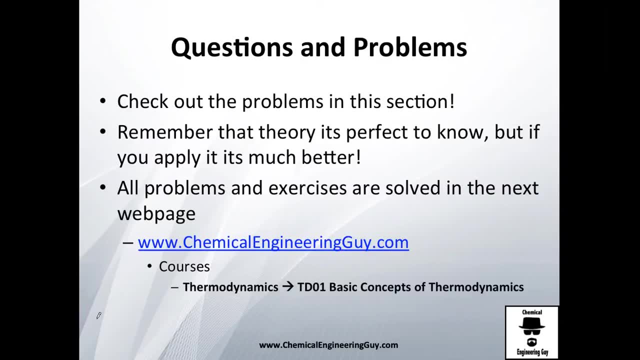 This was about the scale comparisons, So if you want to continue with the serial law of thermodynamics, please go to the next video. So, guys, probably you want to see more exercises, more problems, questions and answers. I got this problem section in my website. 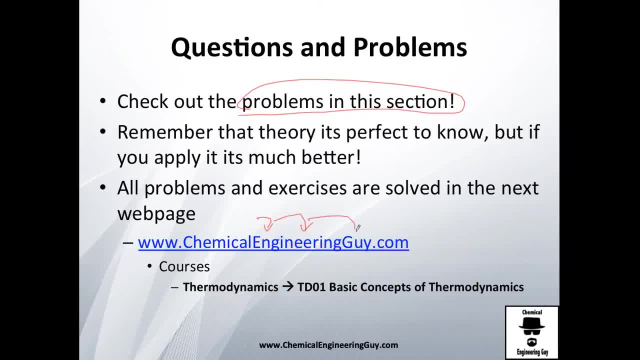 Go check it out. Here is chemical engineering guide dot com. Go to courses and you will find these thermodynamics course. Click on it and check out these block which is TD zero one or TD one, which are the basic concepts of thermodynamics, and going to add some problems, basic problems. 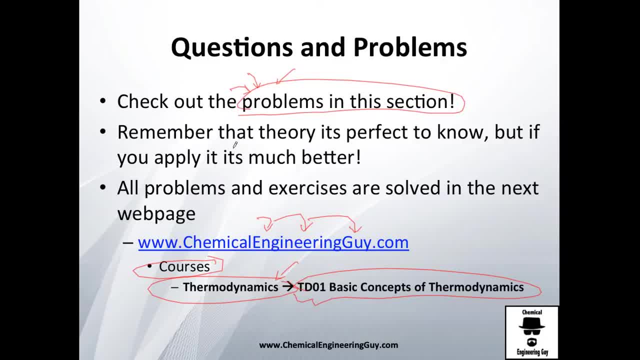 They will help you to start understanding, because you know that theory is perfect to know, But if you apply it it's way better. You even get better basis understand better, you get the ideas faster, you know when you get more theory, you know where it's going to be applied, etc. 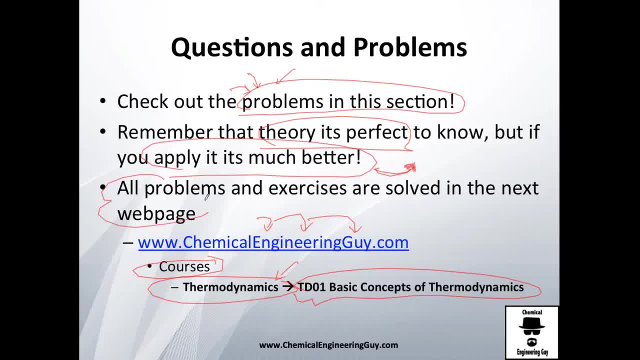 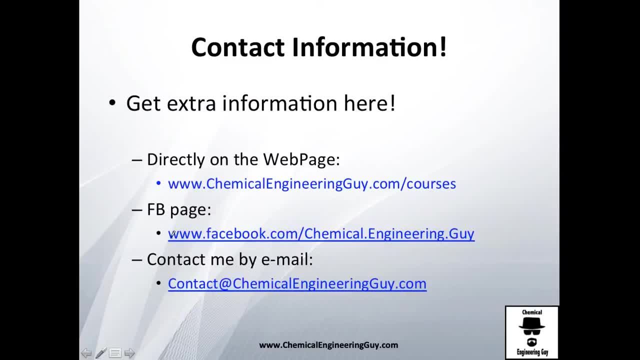 So I totally recommend you. I've got a lot of more material for this course, So I will be pretty happy if you go and check out the course And if you have any type of doubt- comment, doubt, well, Anything- You can send me an email contact at chemical engineering guy dot com, or like my Facebook. 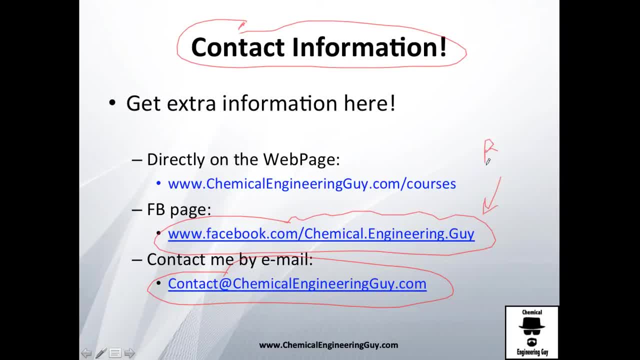 page. I have many stuff. actually. I got some blog stuff and some other funny post- chemical engineering, post engineering in general, how to get the job, etc. And or go directly to my Web page and go to contact- I got A contact form- Or go to courses wherever you want. 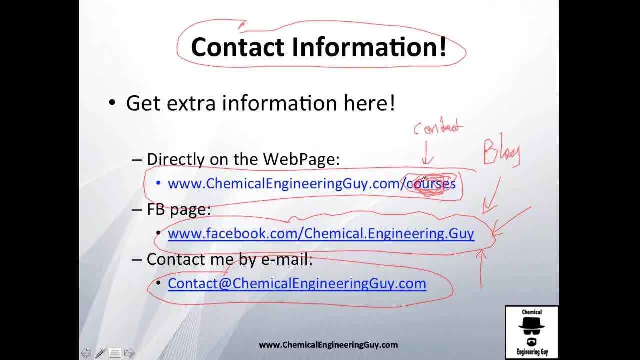 That's what's Everything for these Videos. Thank you for the attention and keep going with the videos, guys. see you in the next one. What's up, guys? It's me- chemical engineering guy. It's very nice to see you all.